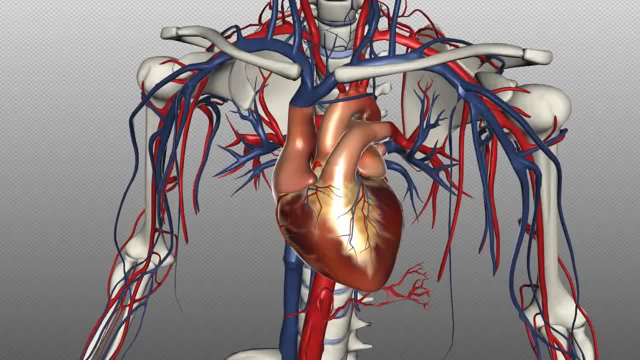 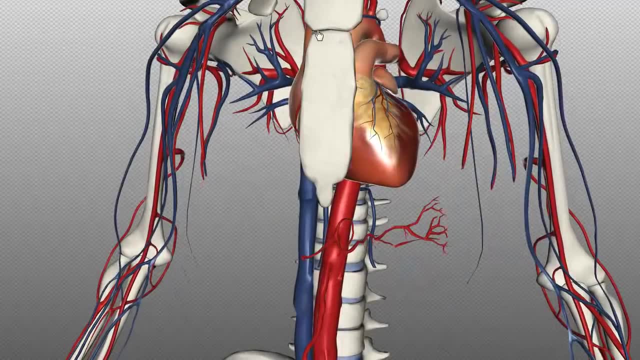 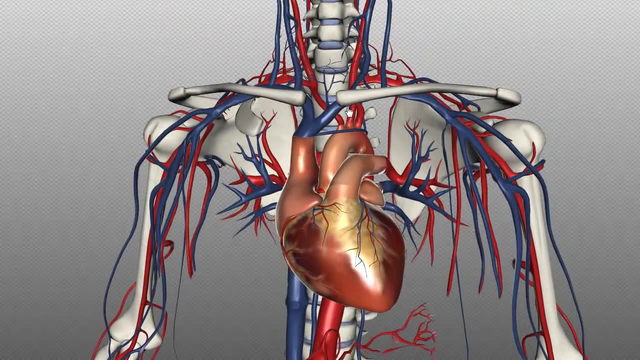 sternum meets the body of the sternum. So if I just show you that quickly, So this junction here is the angle of Lewy, the sternal angle, So that's the level of the disc between T4 and T5.. So the arch of the aorta has three branches coming off which you can see here. So the 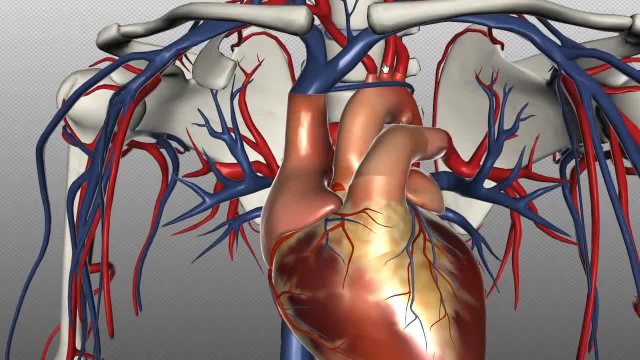 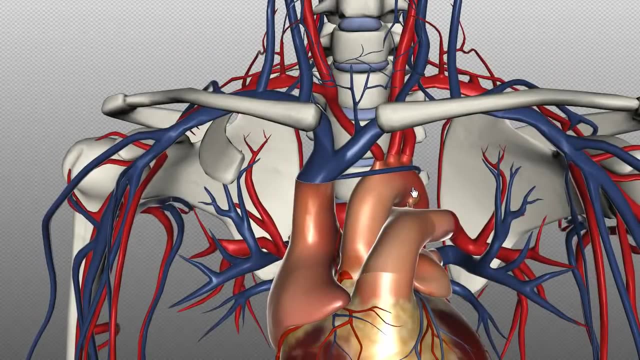 first branch is the brachiocephalic trunk. This second branch in the middle is the left common carotid And this branch here is the left subclavian artery. So you can remember. there's a mnemonic for remembering the branches of the arch of the aorta. So ABCs, as in learning. 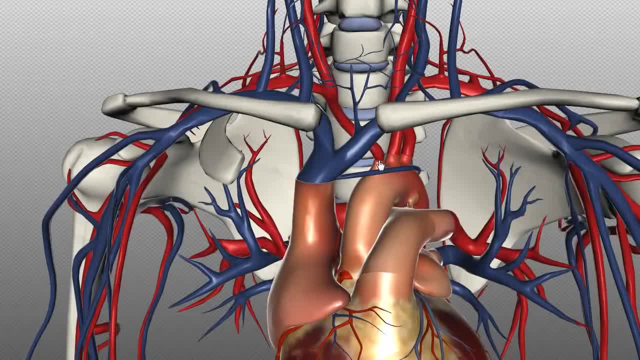 your ABCs. So A aorta, B- bifurcated, C- brachiocephalic trunk, C- common carotid, so the left common carotid, And S- subclavian, so left subclavian. So this branch here, this brachiocephalic trunk, then splits into two branches. You've 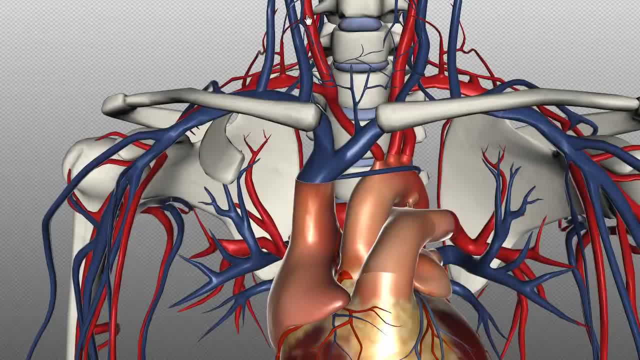 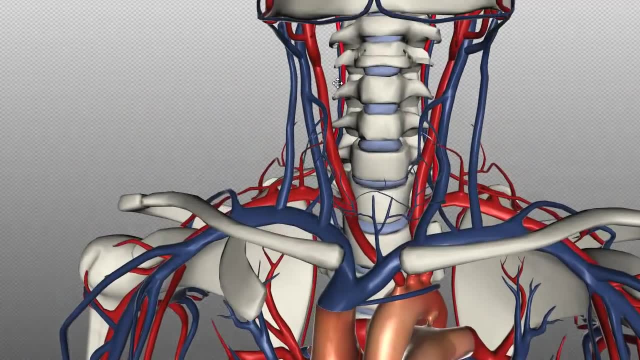 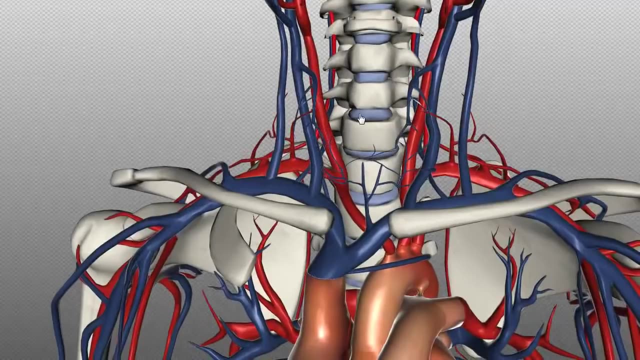 got the right subclavian here and the right common carotid. So just like you've got the left common carotid here, you've got the right common carotid here, Which These two branches off from the brachiocephalic trunk. 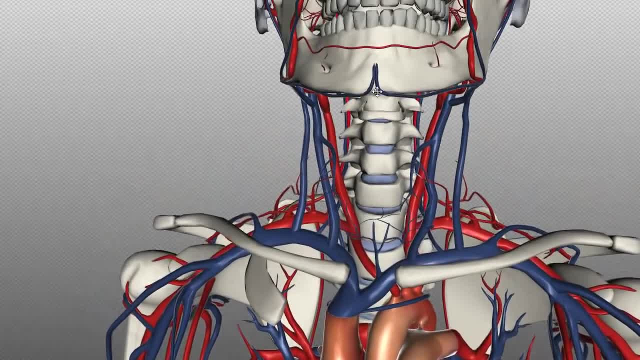 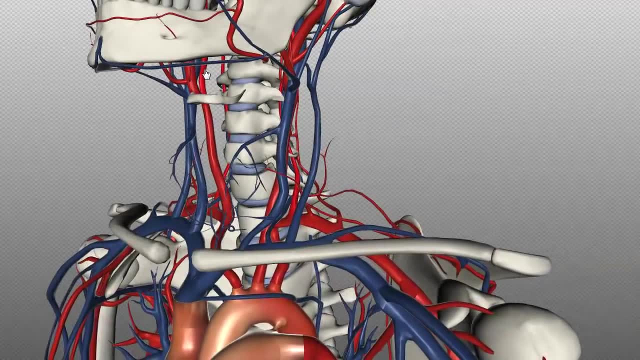 So just following the common carotid arteries up a bit further, they then split into another two branches, So you've got the internal carotid and the external carotid coming off the common carotid artery. The external carotid artery has loads of branches and these supply. 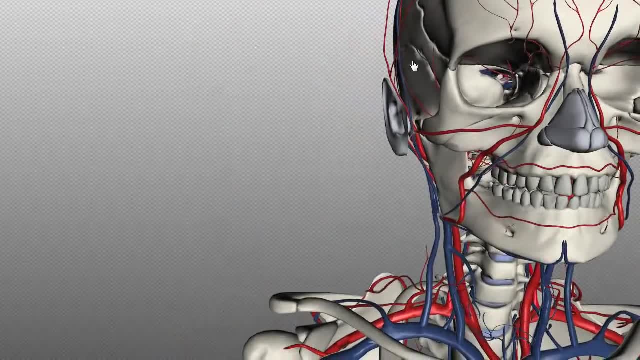 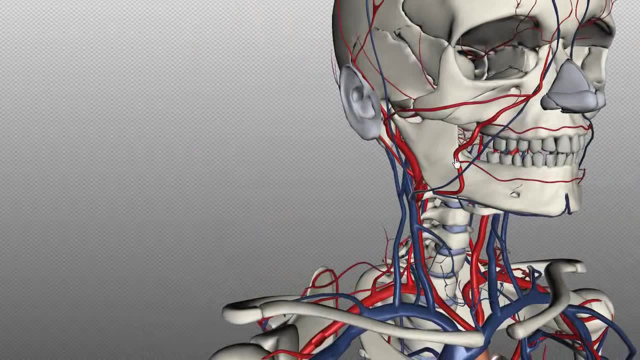 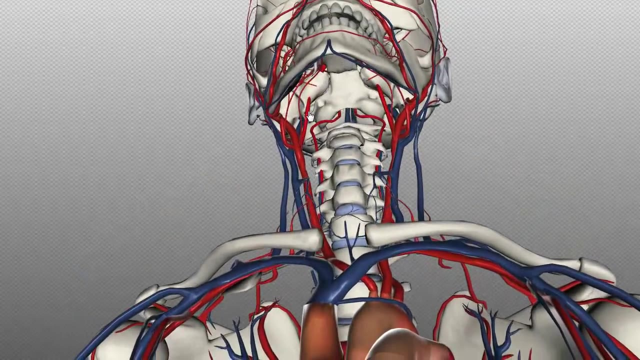 the head and brain, Head and face. So you can see all these arteries on the face. These are branches of the external carotid artery. The internal carotid artery, however, runs straight up to join the base of the brain at the circle of Willis. So this arterial circle at the base of the brain, which 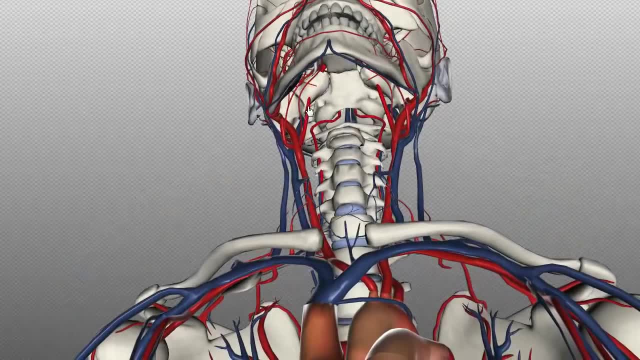 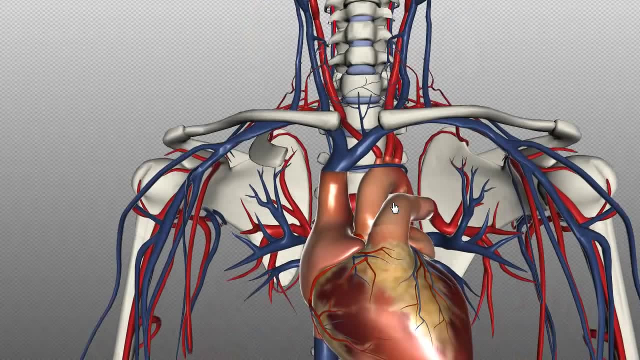 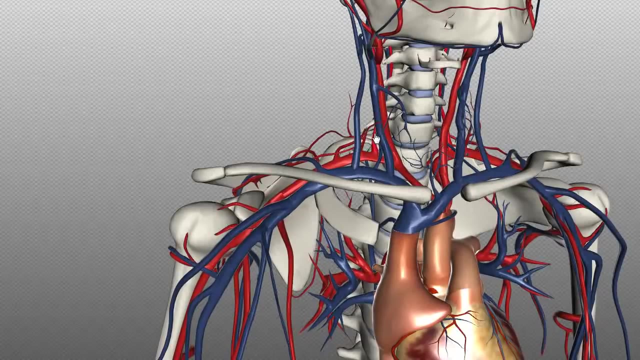 supplies the brain and the internal carotid goes up to meet that. So next, along an important artery to note is this one coming off the subclavian. You've got this on both sides. It's called the vertebral artery. So you've got the common carotid coming. 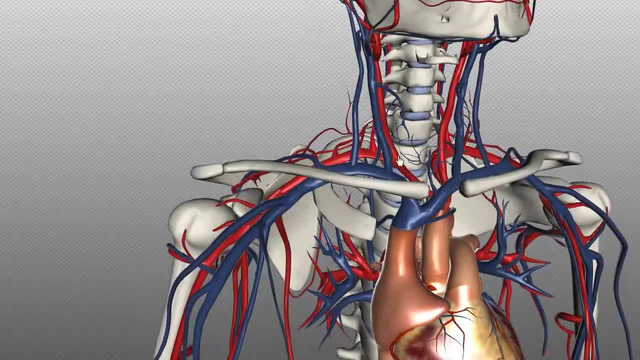 off the brachiocephalic trunk on the right side and you've got the subclavians on either side and you've got the vertebral artery which comes off the subclavian. So you can see the course of this artery Subclavian. 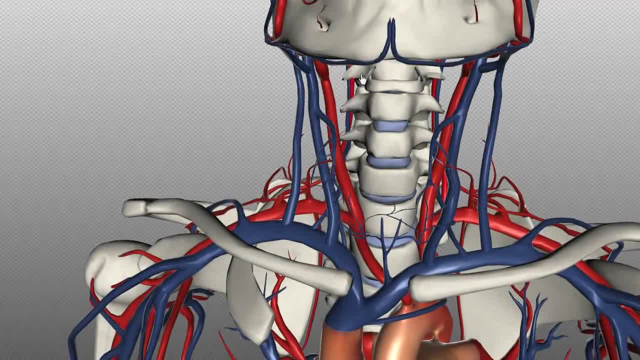 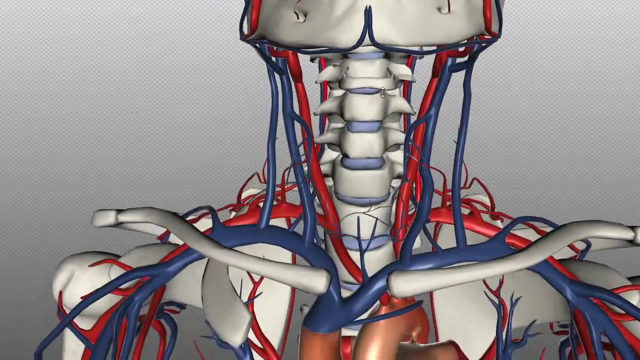 It runs up through the transverse foramen of the cervical vertebra. So you can see this transverse process here and you can see this artery running up alongside the vertebral vein through the transverse foramen. So the vertebral artery runs up and it meets the 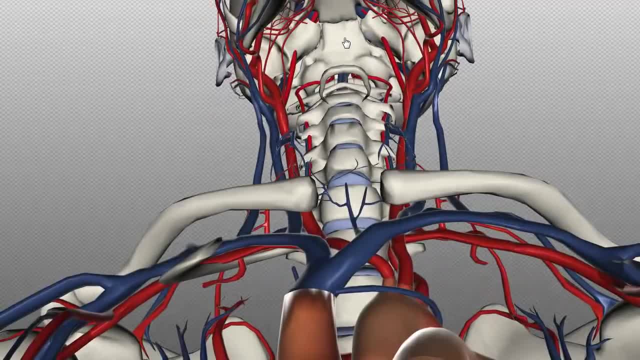 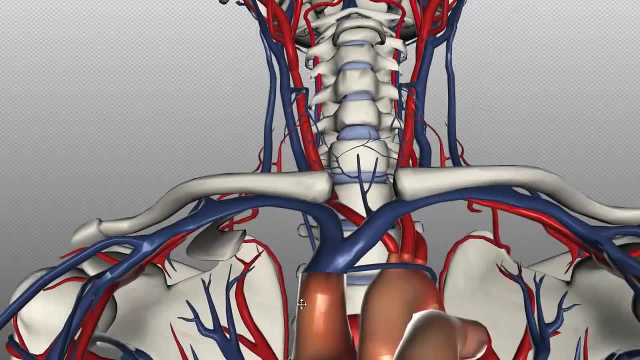 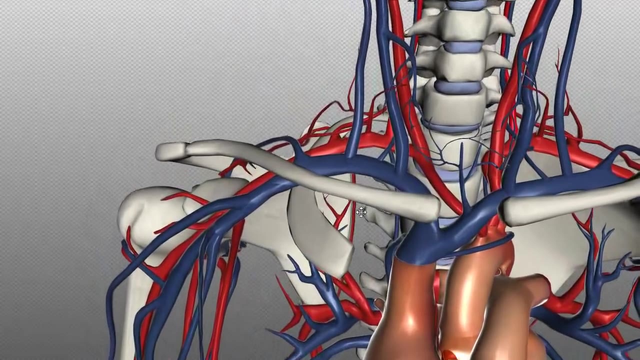 basilar artery to join the circle of Willis and supplies the posterior parts of the brain. So that's the vertebral artery which comes off the subclavian. So I'm just going to follow this course of the subclavian artery and I'll just show you. 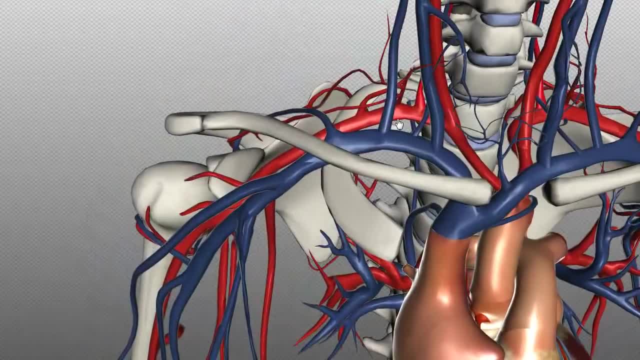 what that extends down to. So the subclavian artery. you can see it running here underneath the clavicle. That's why it's called the subclavian Sub- meaning under Subclavian, Subclavian, Subclavian. 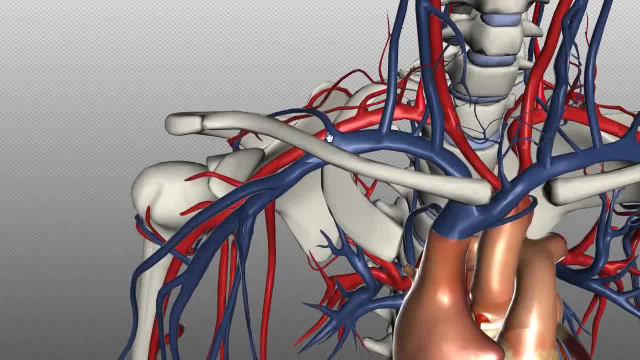 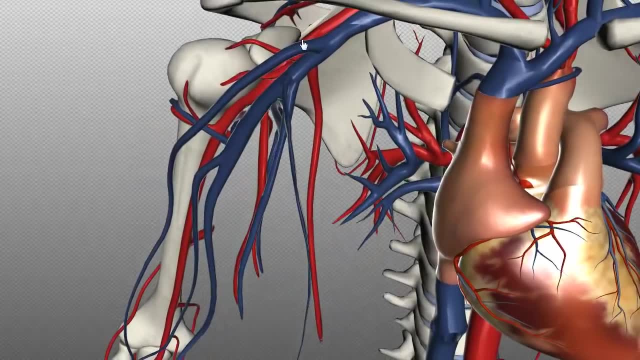 and clavian, referring to the clavicle. So it runs underneath the clavicle, So the subclavian artery becomes the axillary artery, and it becomes the axillary artery at the level of the lateral margin of the first rib. So the axillary artery runs here. 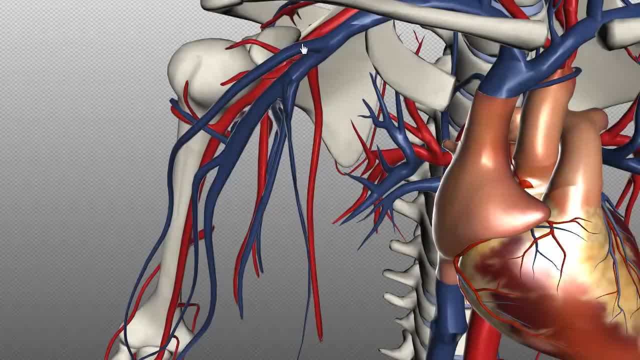 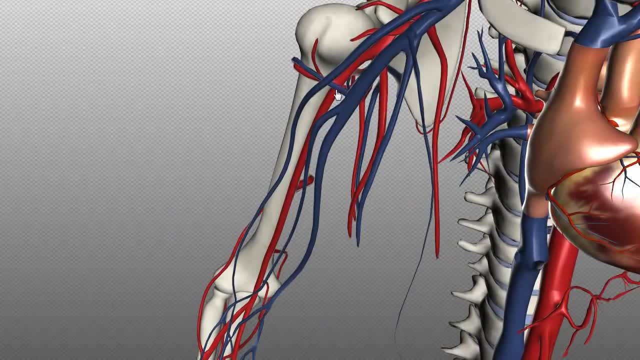 So the axillary refers to the armpit, So it runs in the armpit region. So if we just follow it down, you can see the artery running down the humerus. So this artery is the brachial artery. The brachial artery then splits into two. So you've got 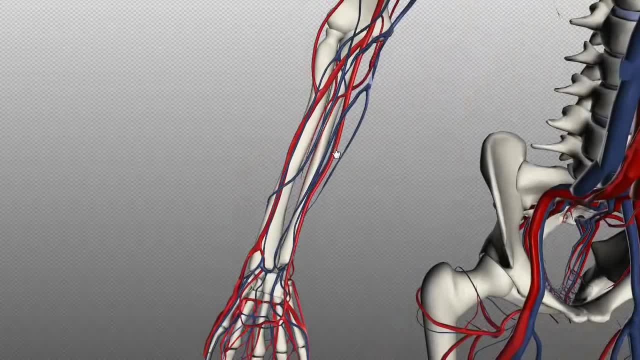 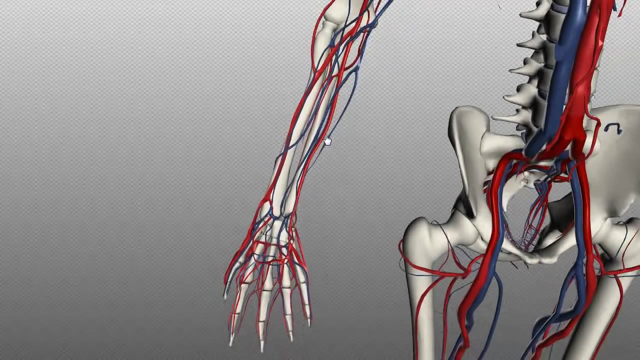 the radial artery and the ulnar artery. Remember the radial is lateral in the anatomical position, So the radius is lateral and the ulnar bone is lateral. So often in clinical medicine you'll hear the words radial and ulnar referring to lateral. 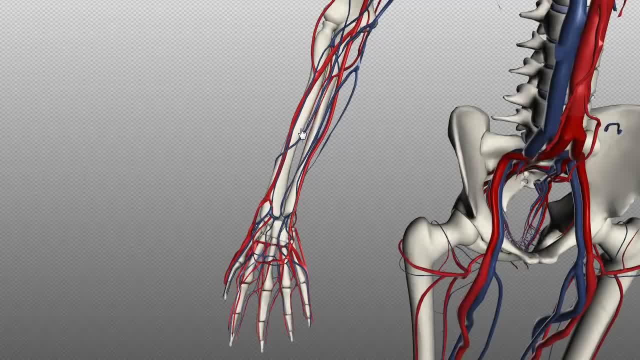 and medial because in the anatomical position the radius is lateral and the ulnar is medial. So the radial artery runs along the radius and is lateral and is on the thumb side, and the ulnar artery runs along the ulnar side and is medial and is on the side of the little. 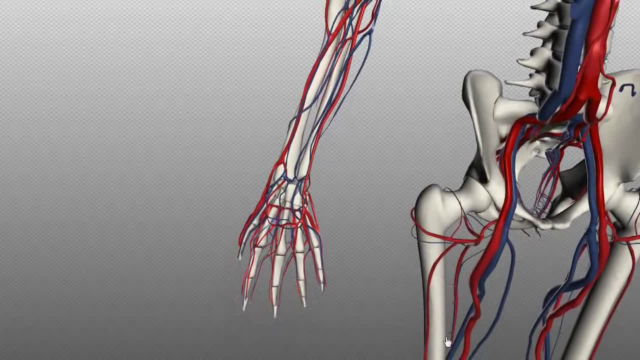 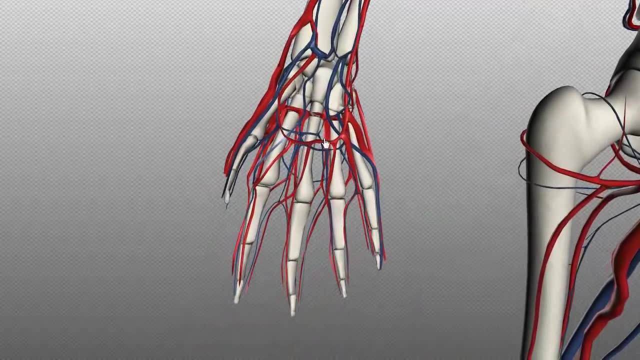 finger. So following the artery a little bit further down, we can see the blood supply of the hand. You can see these arches here. This is the superficial palmar arch and you've got the deep palmar arch. So the superficial arch is obviously close to the surface of the palm. 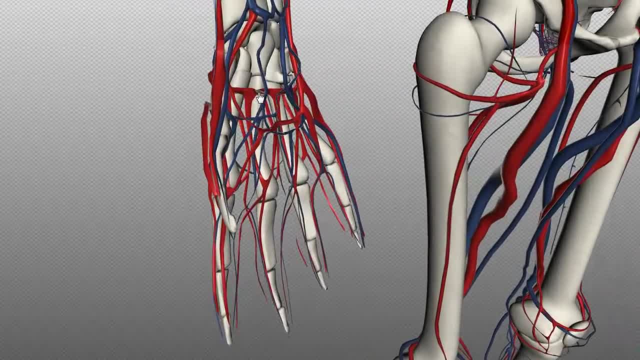 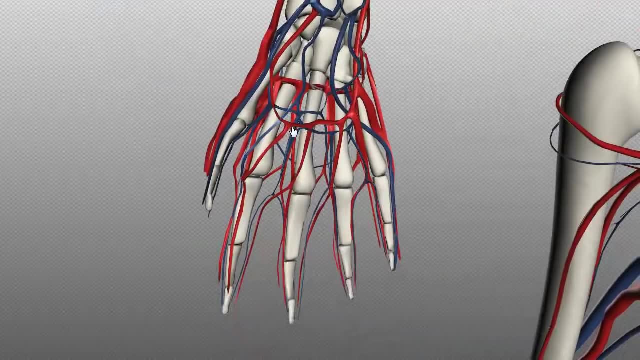 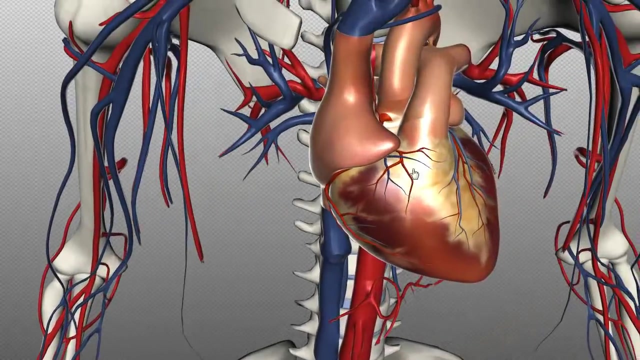 because it's superficial and the deep palmar arch is deeper, obviously. So the superficial arch, as you can see, is further towards the fingertips, So it's more distal and the deep palmar arch is more proximal. So I'm just going to return back to the center of the body, back to the aorta, and we're going. 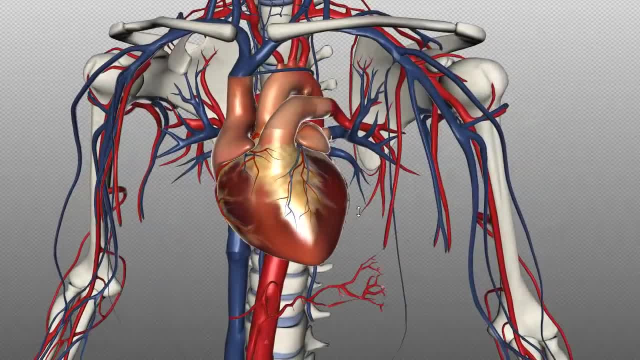 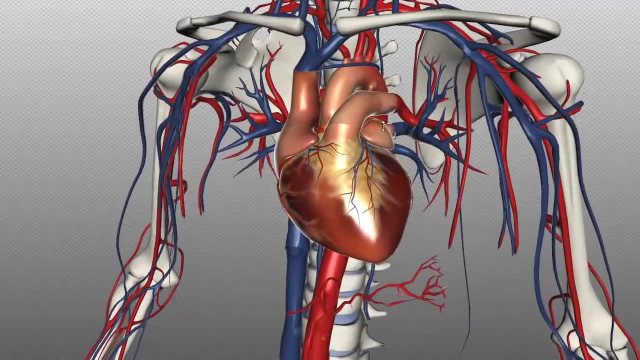 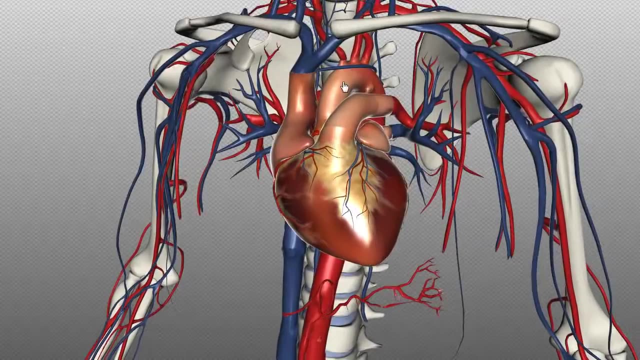 to follow it now down towards the abdomen and lower limbs. End of part 2. The aorta can be divided into five sections. The bit between the heart and this arch is called the ascending aorta. So you've got this ascending portion And then you've got 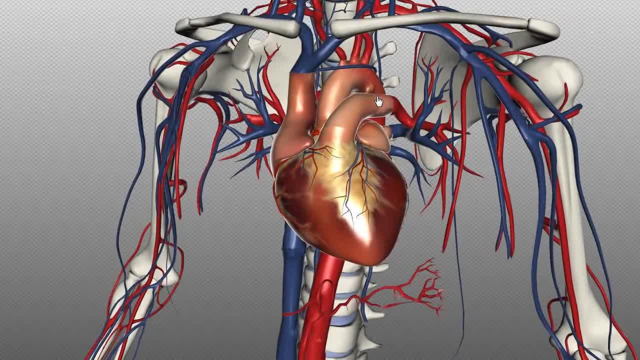 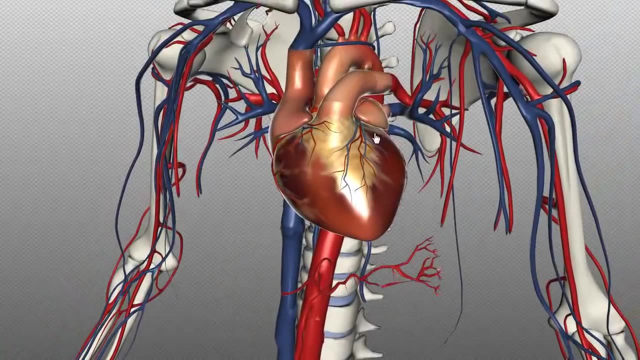 this arch shape. so this is the arch of the aorta, And then you've got the descending aorta, so the section from the arch of the aorta to the point where it divides into the common iliac arteries, so down here. So that's the descending aorta, And then you can divide. 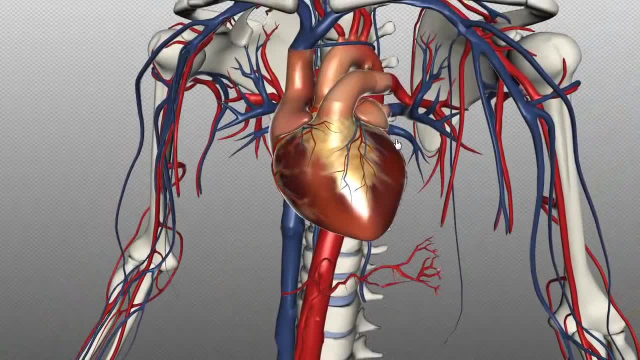 it into thoracic and abdominal aorta. So the thoracic aorta is the section of the aorta which is above the diaphragm.